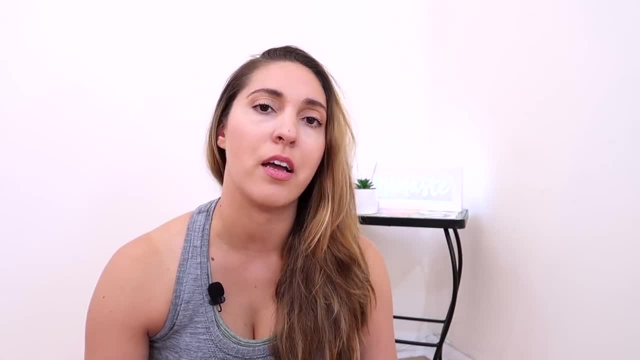 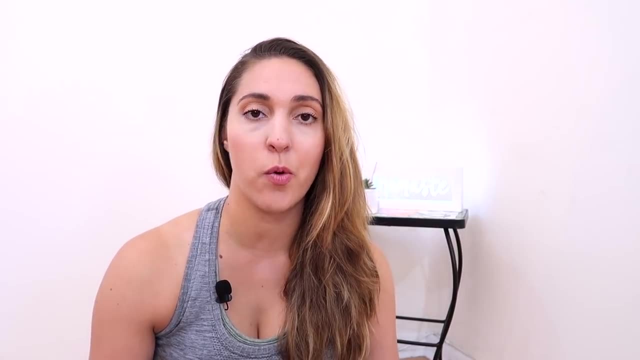 in that video I share how my first experience with yoga. I didn't really like it, and I stopped for a long period of time before I started up again. So these are things that I wish I would have known. So maybe I would have just stuck with it and kept going instead of taking a break in. 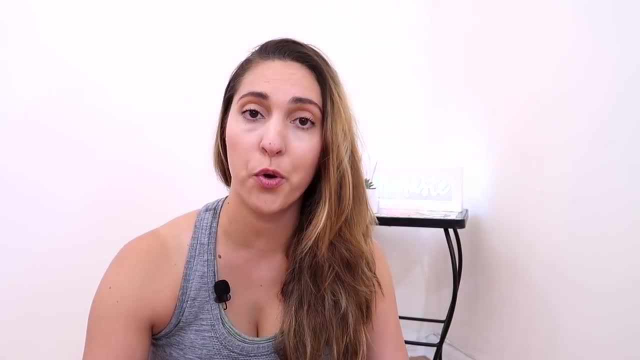 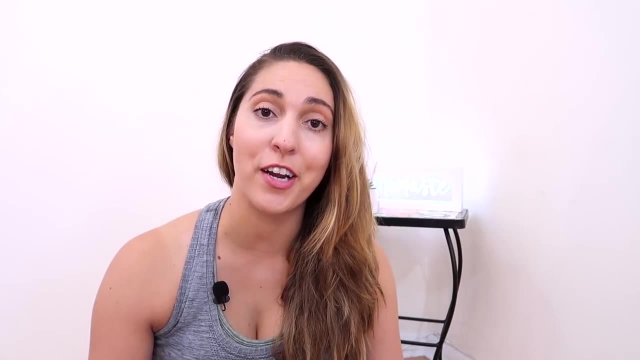 between and just stopping waiting so long to start up again. So if you're a yoga beginner, if you're new to yoga, definitely listen to these tips that I have for you Before we get started. if you are not yet subscribed to this channel, I post two free yoga classes every single week. 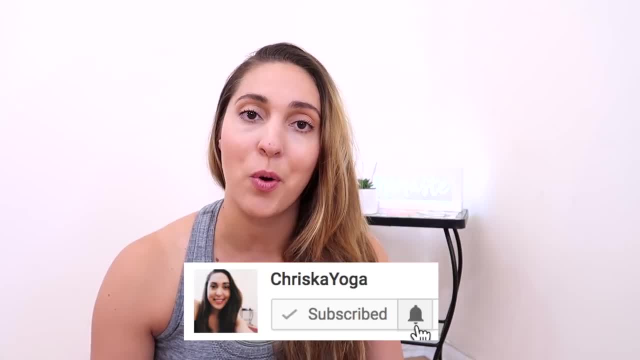 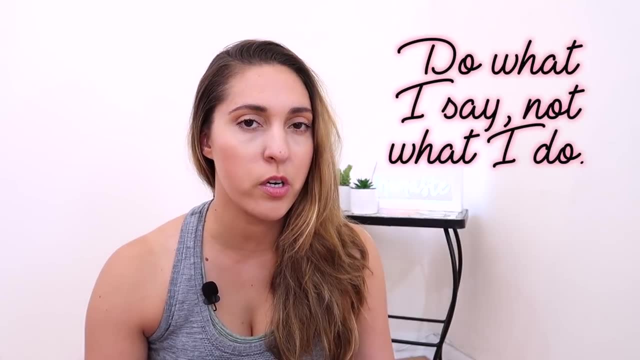 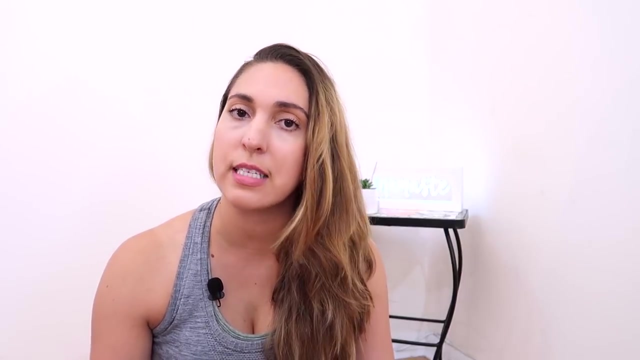 It is completely free. So make sure to subscribe, and I would love to have you as a subscriber. So let's get into my five tips for yoga beginners. Number one is: listen to my words instead of looking at my body. So you can look at my body in the pose when I'm demonstrating, for an example, but I would say, listen to my 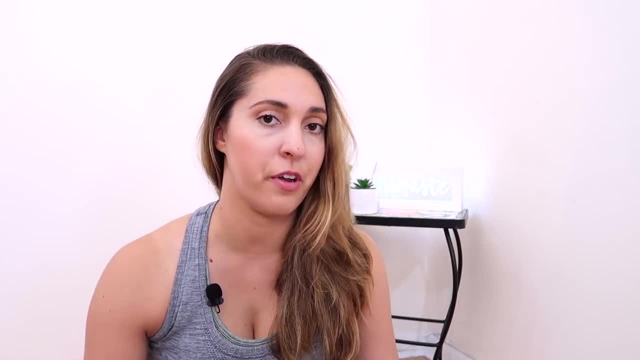 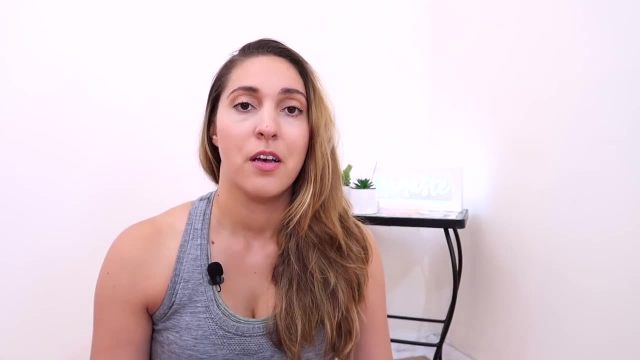 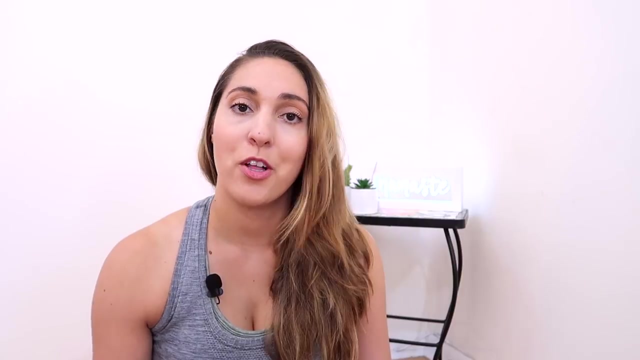 instructions more carefully, because I'm not perfect, My body is not perfectly aligned and my body is still working towards more flexibility, more strength. I do have some flexibility and I do have some strength, but it took me a long time to get there and it's going to take me a long time to get even better, So I know how. 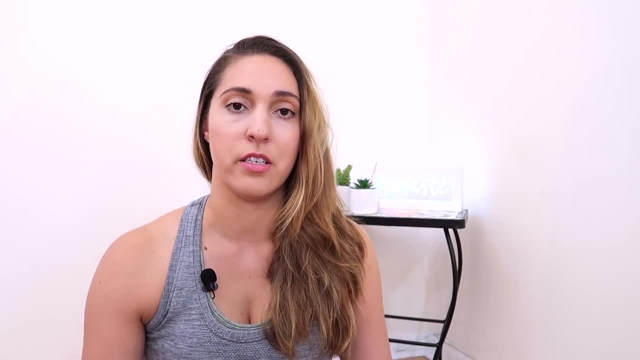 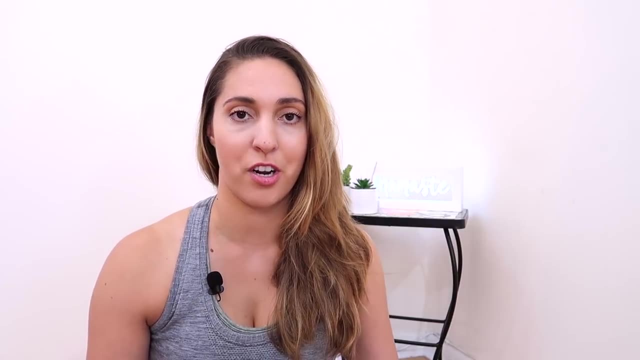 the body needs to be in order to stay safe and achieve the pose correctly, in the right way. And I think about what I say when I instruct you into a yoga pose. I'm saying this as a yoga teacher When I am giving yoga instructions, yoga asana. 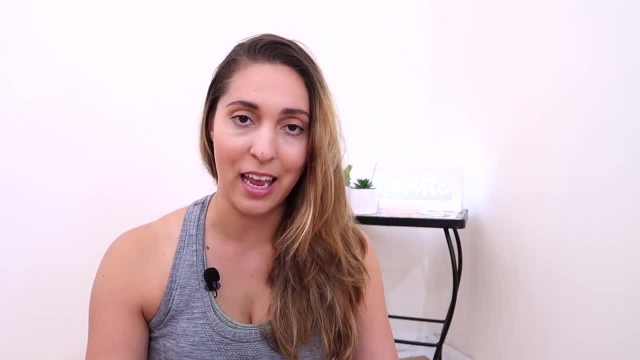 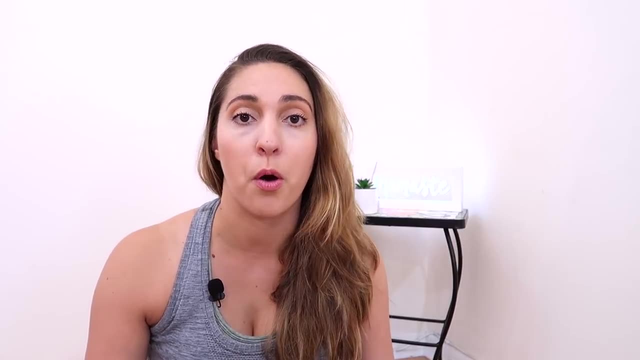 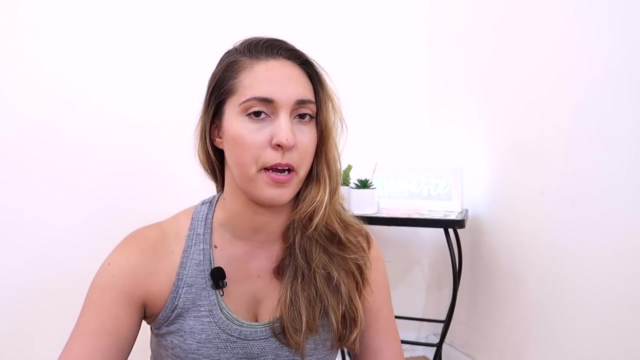 I put a lot of thought into what I'm saying and the instructions are carefully constructed so that you are able to achieve your optimal yoga pose. Sometimes my body may not look the way your body is going to look, and that's totally fine, which brings me to my next point a little bit. 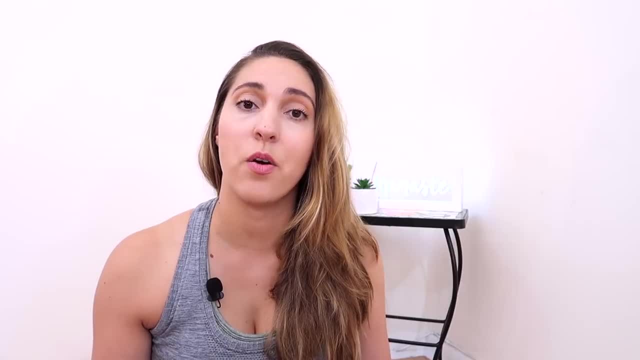 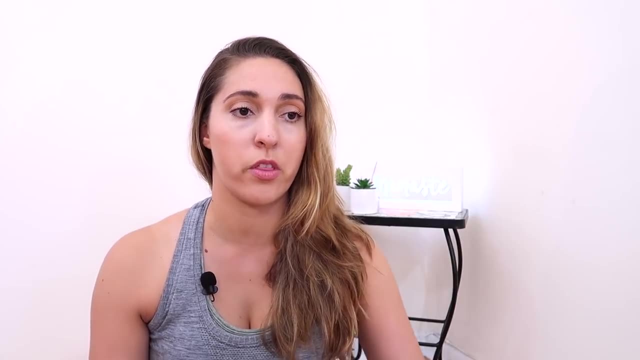 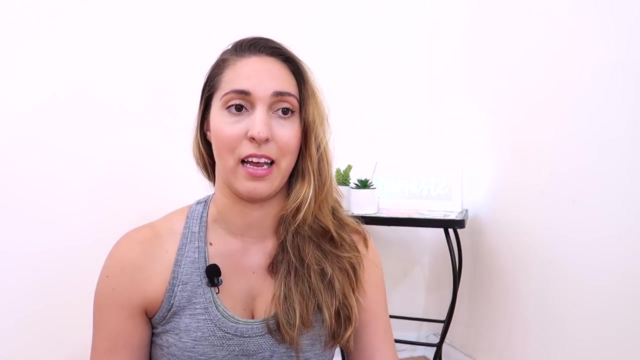 But just hold on for a second with that. Another point to this is that I notice a lot of students when I'm teaching live classes. they're in their head way too much. I can be looking straight at someone with their left eye, my left arm raised, and I can say: raise your right arm. They are just so focused on what's going on in their head and I can just repeat that phrase. 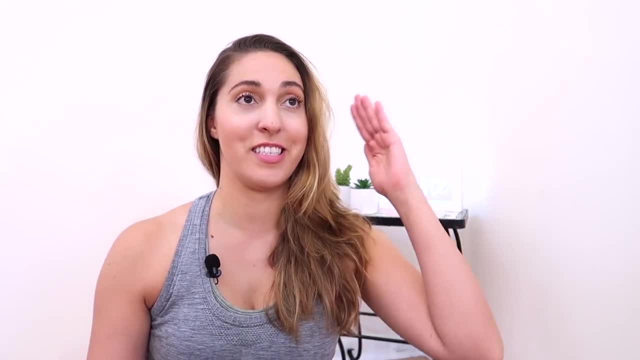 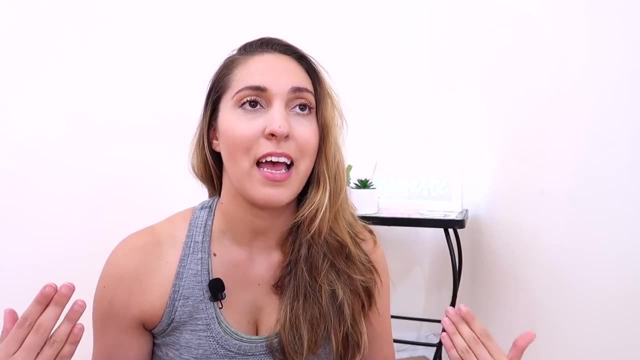 raise your right arm, raise your right arm, raise your right arm, and they're still with that left arm straight up above their head. It's just so funny how- and I do this as well- we're just always in our head and we're focused on what's going on in our mind and we're so focused on other things. 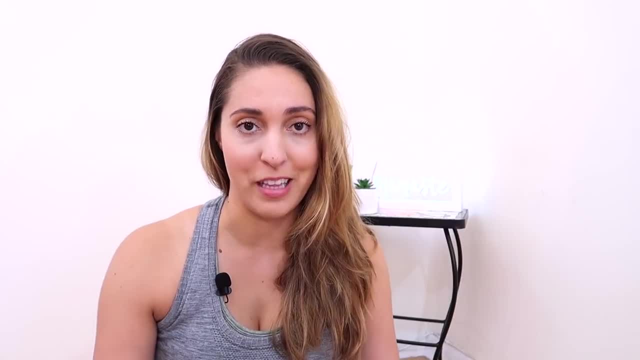 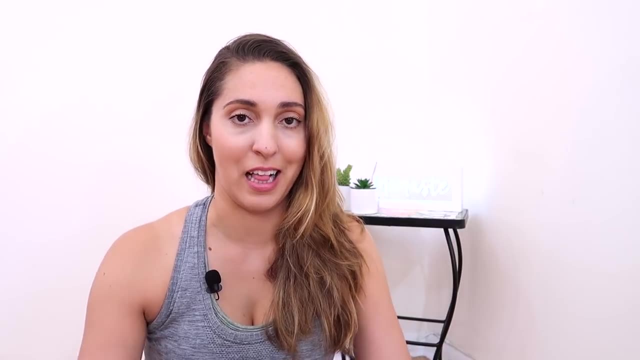 When we're in a yoga class, we need to listen a little bit more carefully to the instructions of the yoga teacher. We all do it. as I said, I do this as well when I am a student in class, But it is super important, especially if you're a yoga beginner just learning the poses. 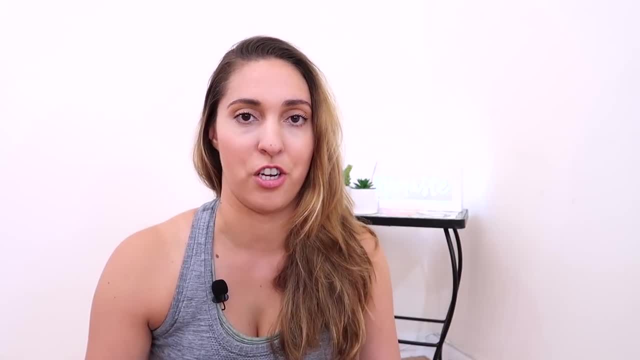 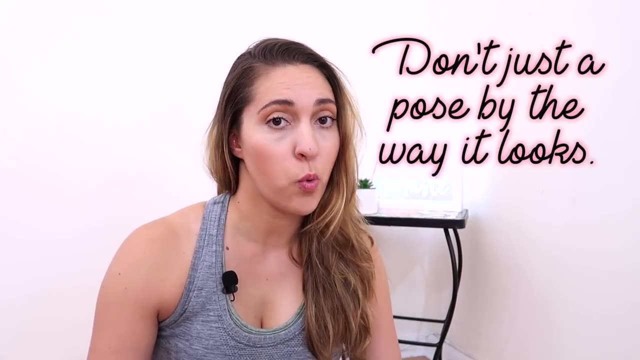 Keep those ears peeled and listen really carefully to the instructions of your yoga teacher. My number two tip is: don't judge a pose by the way it looks. This could go two ways. You could look at a pose and say that is way too hard and I'm never going to do that. 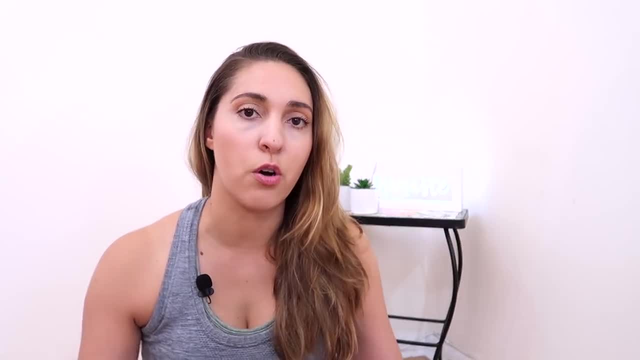 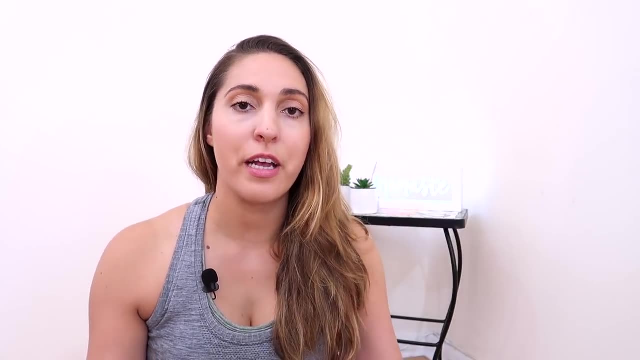 Or you can look at a pose and say: that is super easy, Let's go for it, I'm ready. that looks too easy even. But poses can be deceiving and, as we all know the phrase don't judge a book by its cover. 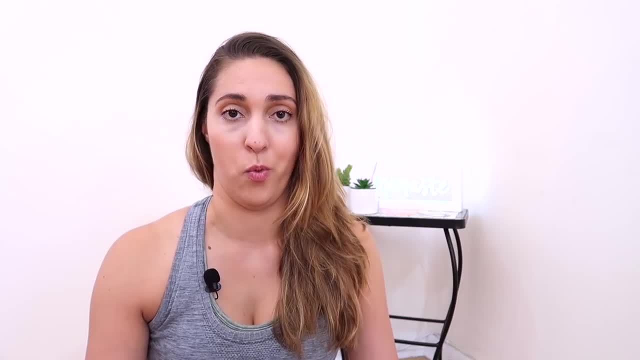 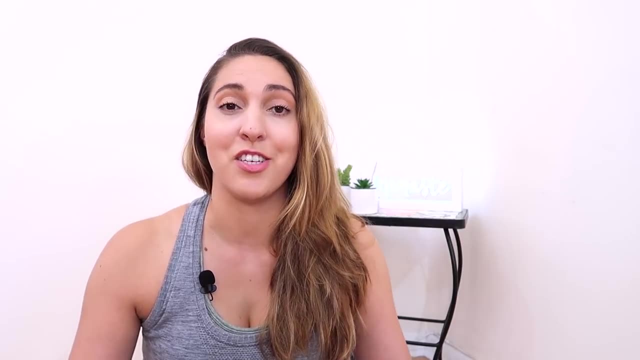 the same goes for yoga poses. Don't judge a yoga pose by the way it looks, especially by the way it looks on someone else's body who is completely different to you, or by the way it looks in an illustration you might see online or in a book. 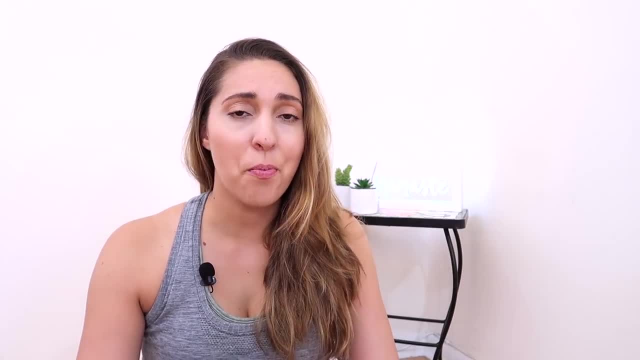 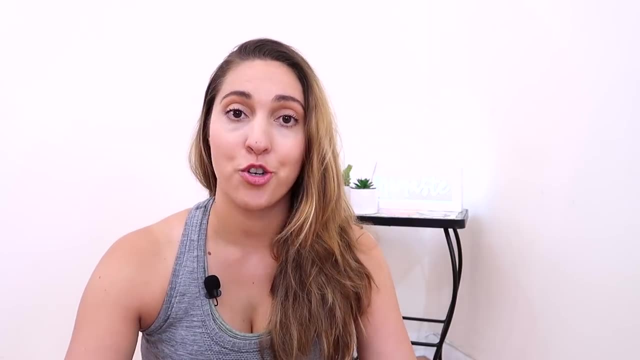 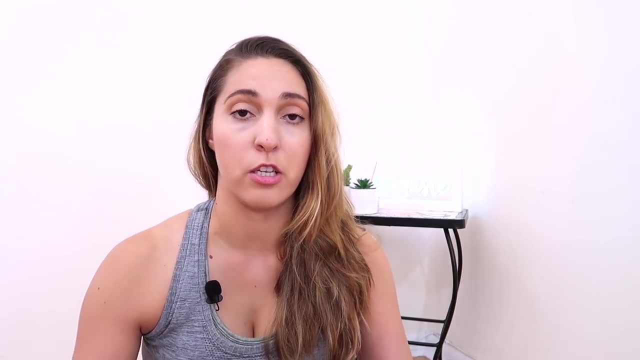 Illustrations are not always accurate in terms of anatomy, and other people's bodies will often not look the same. So don't judge a yoga pose by the way it looks. Give it a try, try it out for yourself. You can look up pose tutorials online. you can reference a book, the instructions of 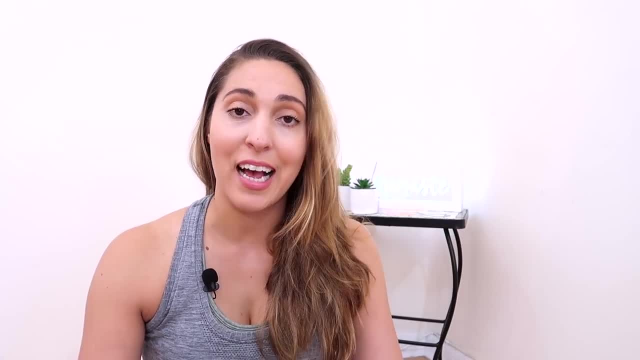 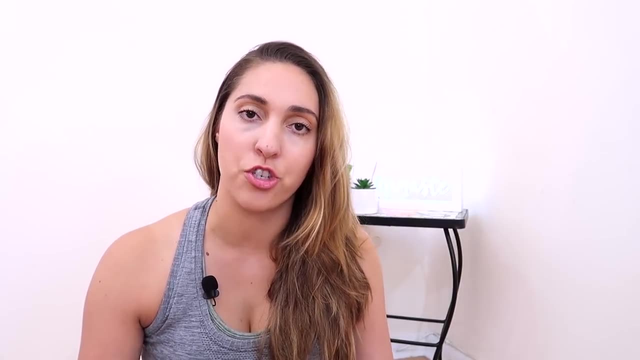 a book and try it out for yourself. You can ask a yoga teacher to instruct you on how to do the pose and try it out for yourself before you make a judgment about it. Which brings me to my next point, which is my number three tip. 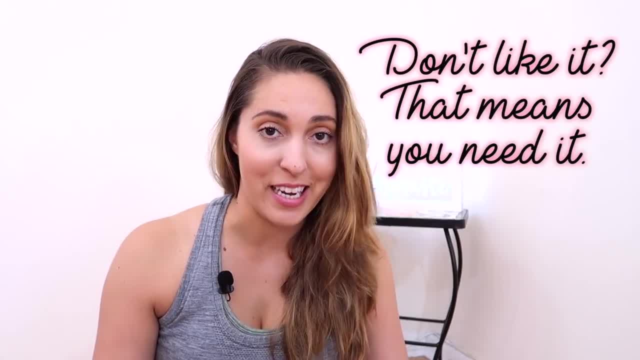 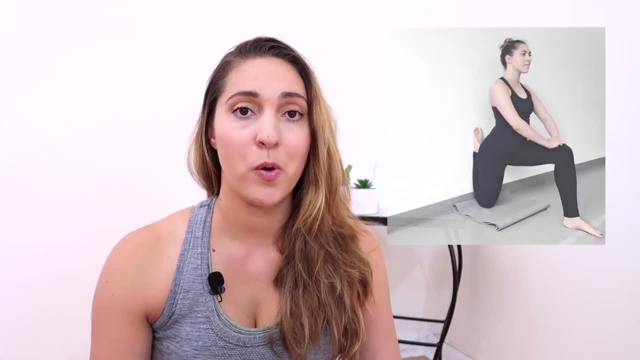 So you don't like the yoga pose, that means that you need it. For instance, there's a pose called King Arthur. I discussed this on my Instagram a little while ago. There's a pose called King Arthur that I've done a tutorial about on this channel a few. 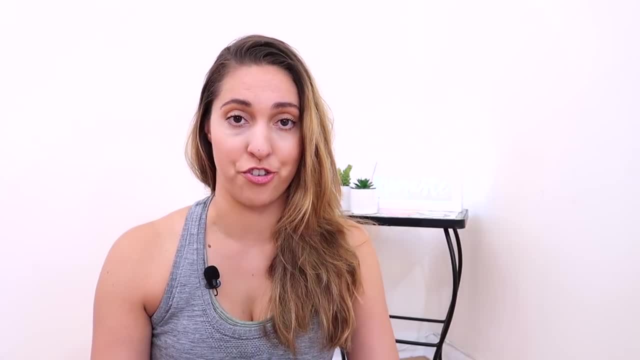 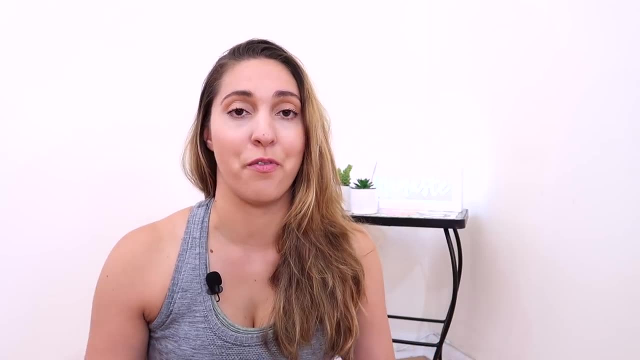 years ago now. It is a very intense and deep quad stretch and sitting down all day. especially now I'm sitting down on my computer a lot, my quads and my hip flexors are very tight. King Arthur is really tough for me. 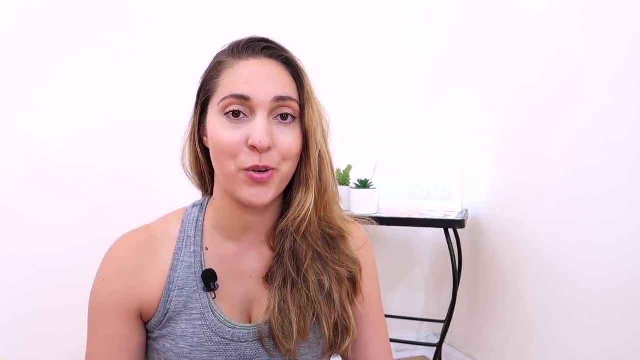 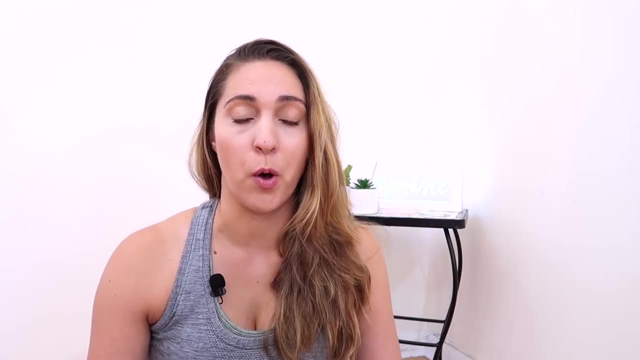 I hate doing that pose. it is something that I dread doing, and I don't do it nearly as often as I should. But since I know that I feel this way about this pose, I also know that this is a pose that I really need the most. 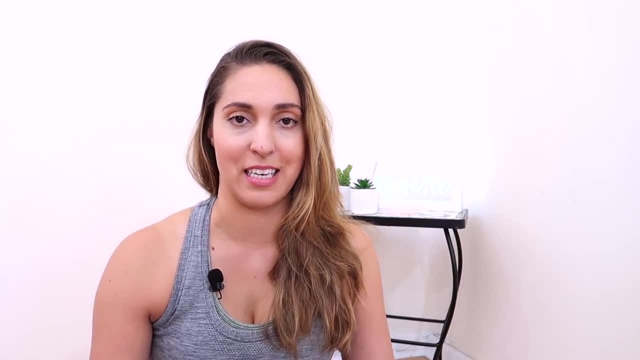 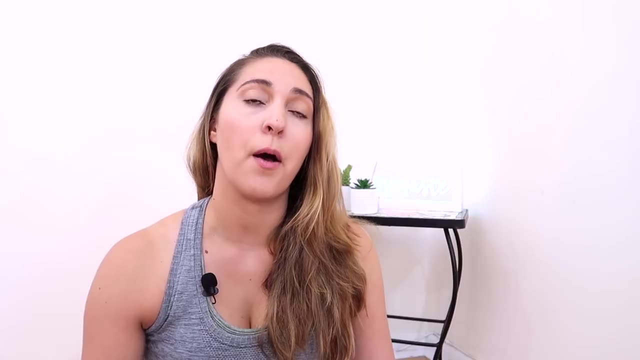 This is something that my body is in need of. my body is in need of more flexibility and openness and ease in my hip flexors and in my quads, So this is definitely a pose that I should be doing more often. So this is just an example. 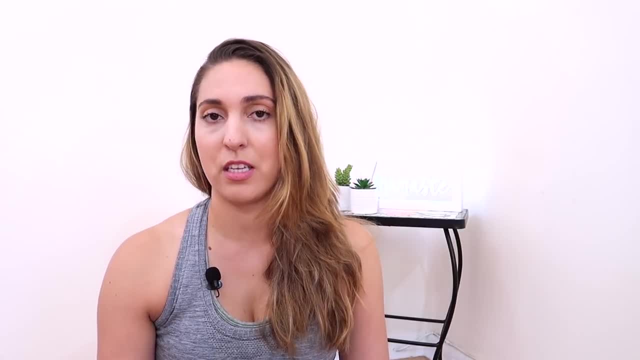 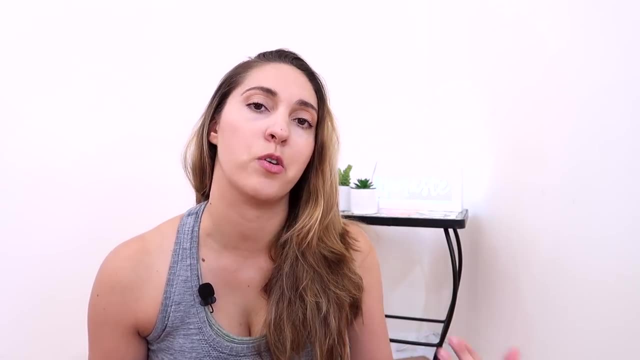 Everyone is tight in different places. everyone is more flexible in different places, so some poses will be a little bit easier for you and some poses will be a little bit more challenging. I would say the ones that are more challenging are the ones, generally, that you need to practice. 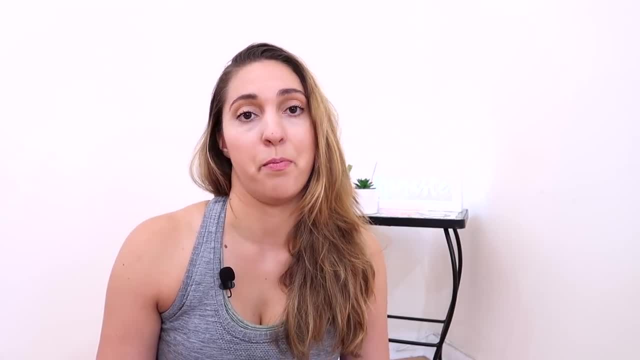 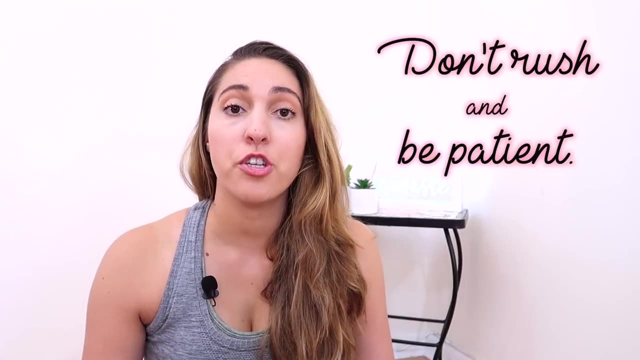 the most, and they may turn out to be your favorite poses. My number four tip for yoga beginners is: don't rush and be patient. So, especially when you're a yoga beginner, You might not be able to do that. You might not be able to do that. 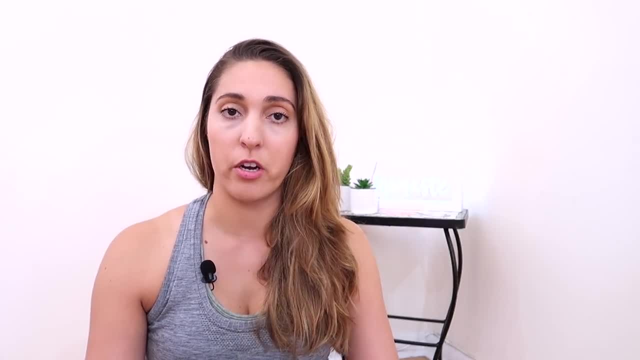 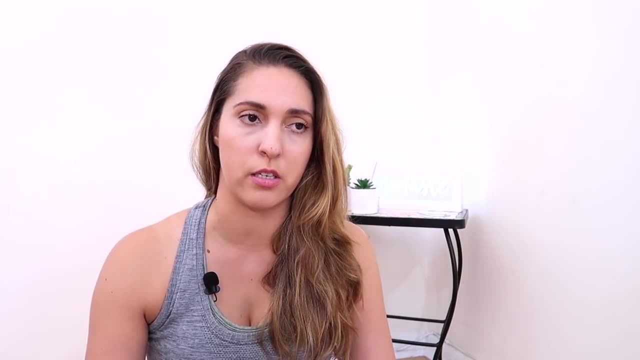 You might not be accustomed to holding poses for long periods of time. That's why in my beginners poses I like to add some movement a little bit. especially in the warrior poses I add a modification, add some dynamic movement to make it a little bit easier to hold the. 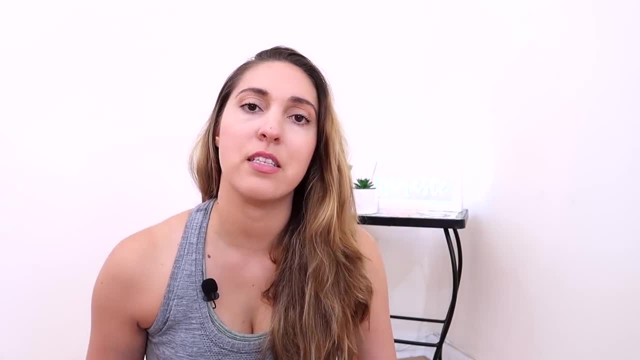 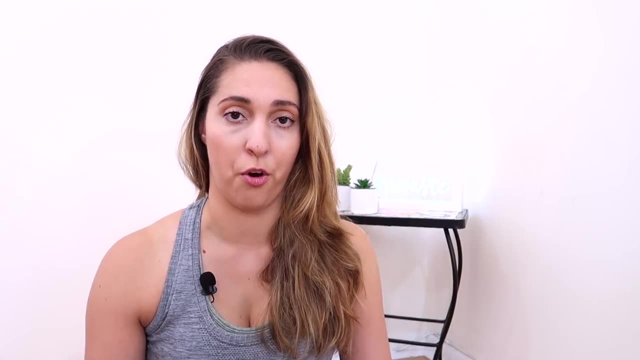 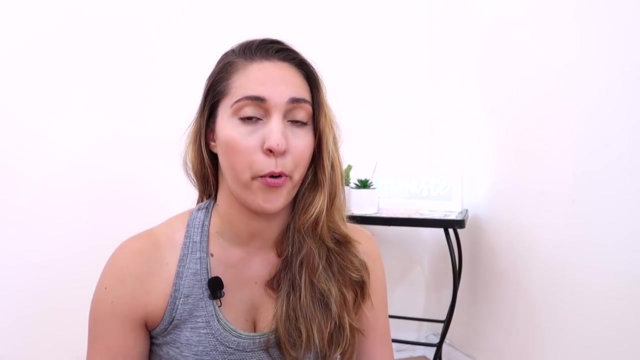 pose or to maintain the pose. But when you get a little bit more advanced- maybe at the strong beginner or intermediate level- you need to get a little bit more accustomed to holding the poses for longer periods of time. beginner: it's great to pay attention to when you want to rush out of a yoga pose. try to be patient. 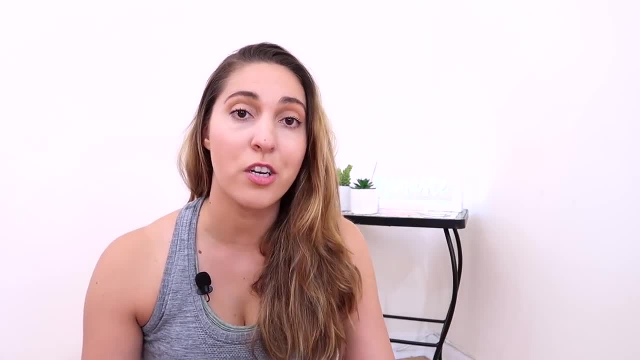 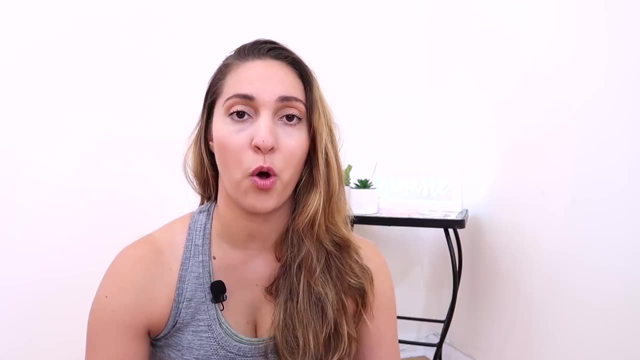 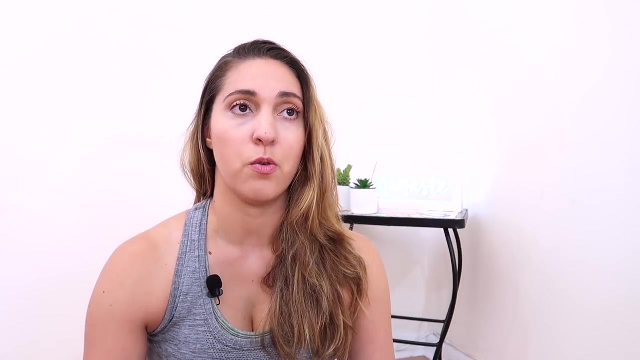 and hold it for just a bit longer than you normally would want to. some tips to being a little bit more patient with yourself is focusing on your breath, drawing your attention away from the fact that you're uncomfortable or you're feeling more fatigued, maybe, and trying to focus on your. 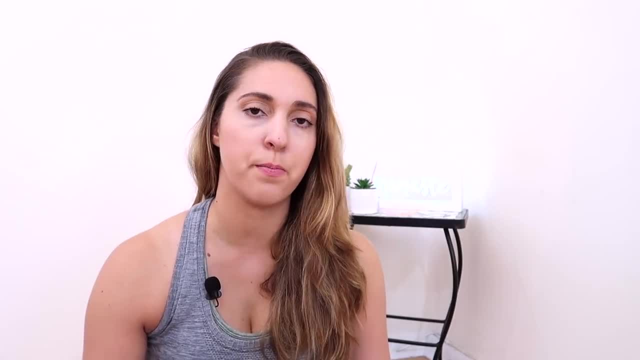 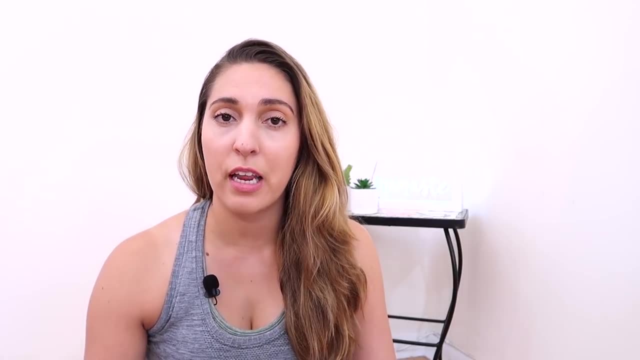 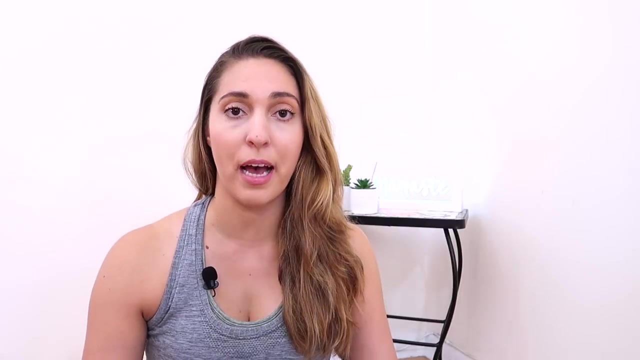 breathing instead. also, another aspect of this tip is be patient with yourself in terms of achieving certain yoga poses, for instance. sometimes we might get frustrated maybe, let's say, if we're trying to achieve handstand or headstand or any of the inversions or deeper back bends, and we might 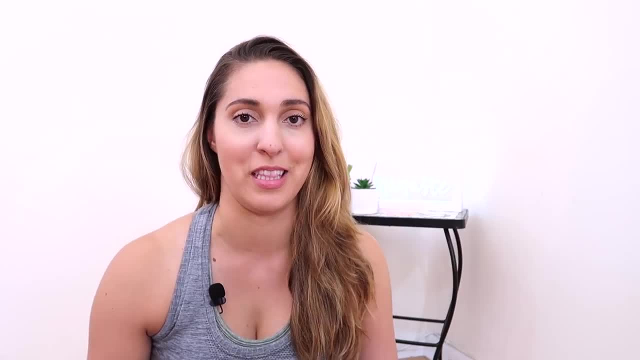 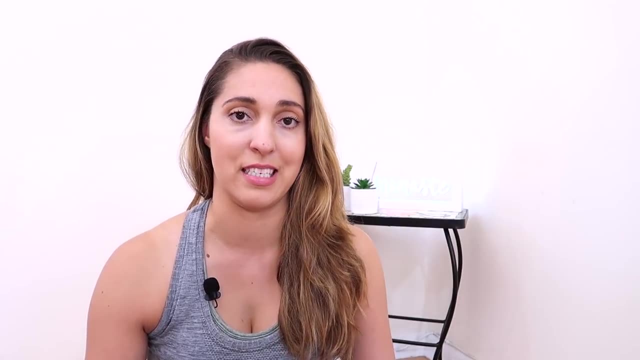 be discouraged because they're not coming as fast as we would like them to come. i would just say: be a little bit more patient with yourself. i know it's frustrating and everyone's body is different, but be patient with yourself and be patient with yourself and be patient with yourself. 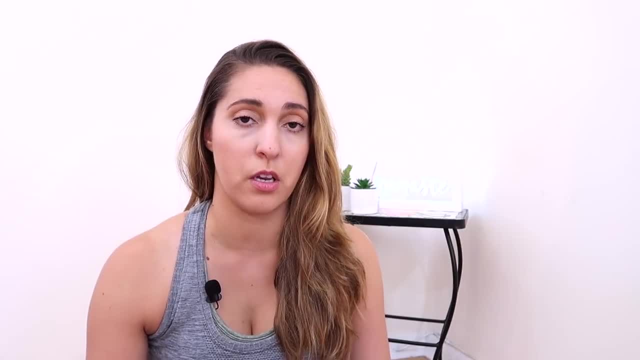 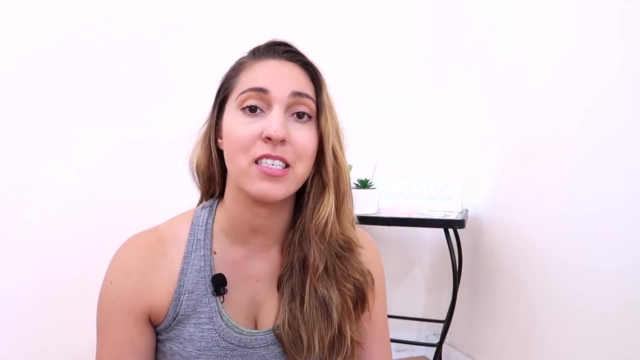 different, so it might take you a little bit longer to achieve this pose than you would like to. but i would just say: be persistent, keep practicing and be patient with yourself and don't rush into anything, because this could cause injury. so you want to be safe and you want. 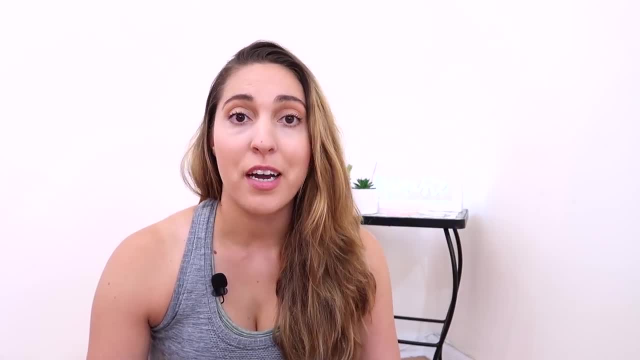 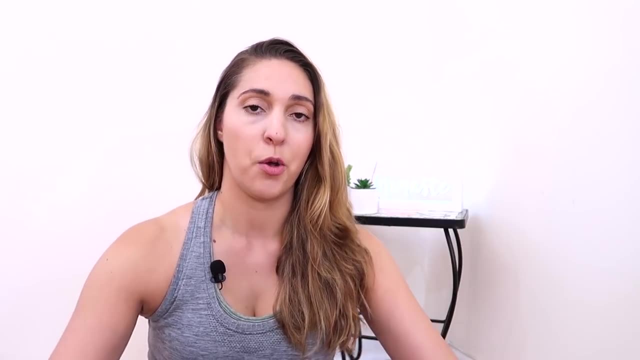 to ease yourself into a yoga pose. perhaps, if you're trying to do handstand, you might not be quite ready to go upside down and support all of your weight with just your hands and arms. you might need to build some more upper body strength and do some more of the 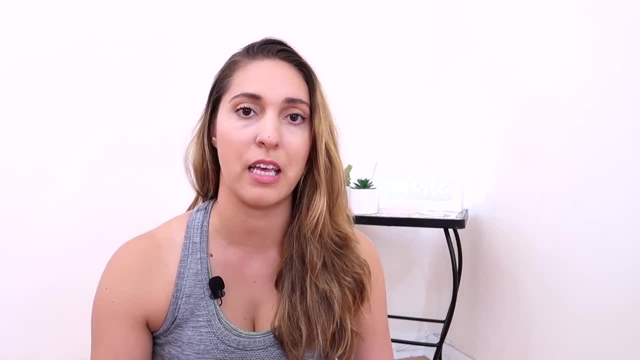 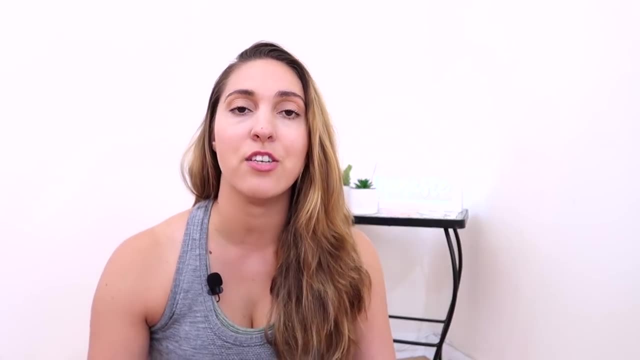 practice. you might need to build some more upper body strength and do some more of the practice preparatory poses in order to achieve that pose. ultimately, you just need to ease yourself into it and be more patient with yourself, you'll. you will get there eventually. just be patient. 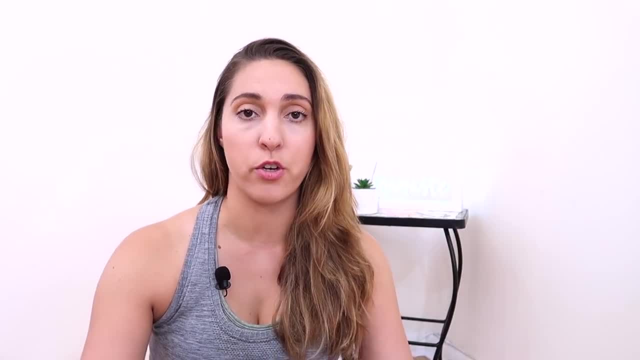 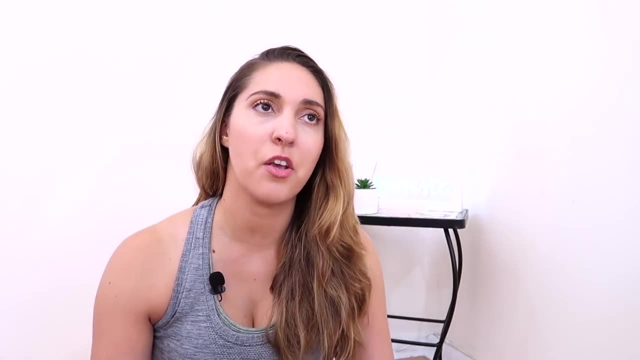 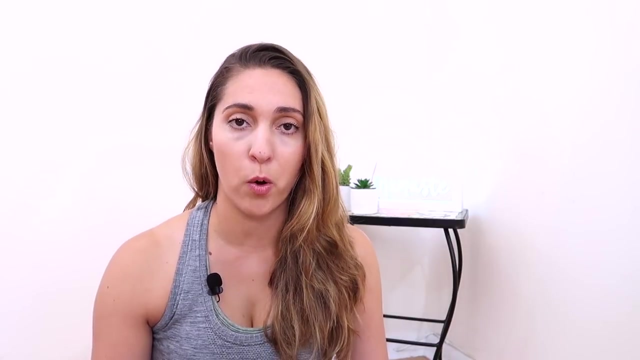 and my final number five tip for yoga beginners is to start out at home. everyone is different, but if you're new to yoga it is likely that you might be a bit self-conscious. you might not want to jump right into a big group yoga class if you aren't familiar with the poses. 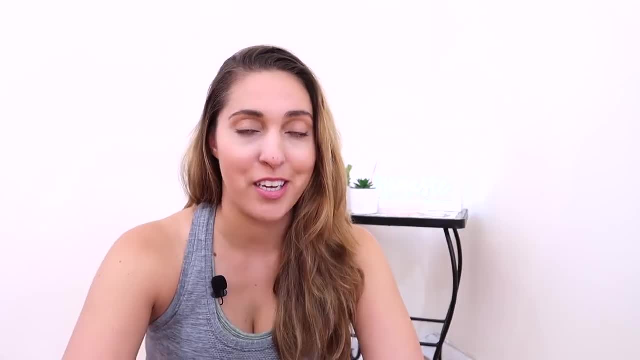 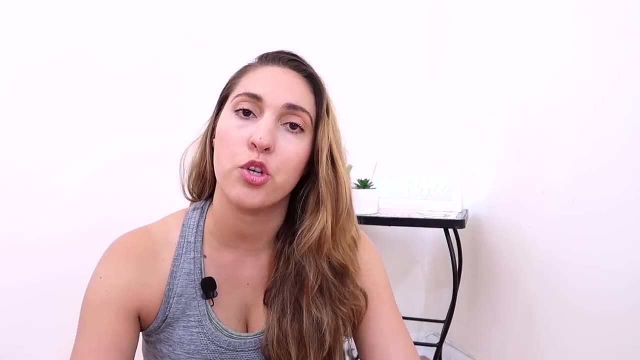 yet. so practicing yoga at home might be a great way to start. another way that you can do this if you're feeling self-conscious, is to get a yoga private lesson. most yoga studios- their teachers- offer private lessons. you can find tons of yoga teachers in your area that offer private. 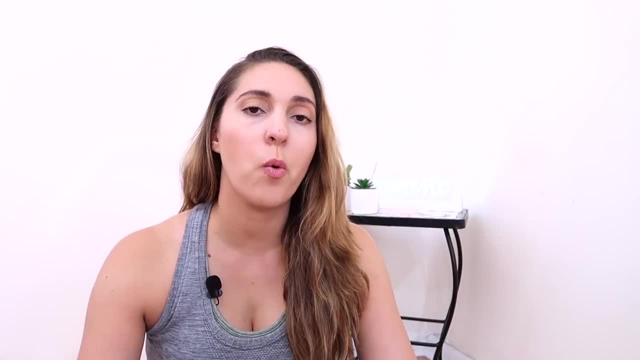 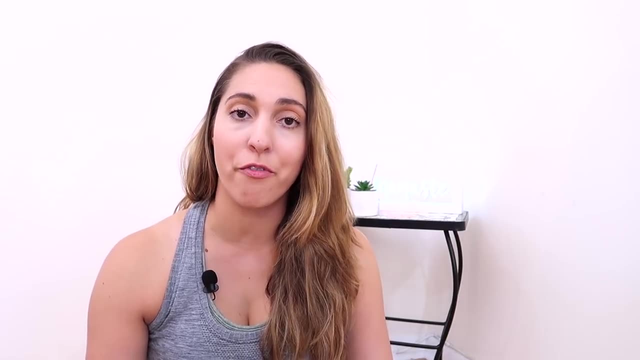 lessons by just doing a simple google search. private lessons are always a great way to start out if you're able to. they can be a bit pricier, which is why practicing at home with yoga videos on youtube or even yoga is always a good way to start out as a yoga coach if you're able to get a. 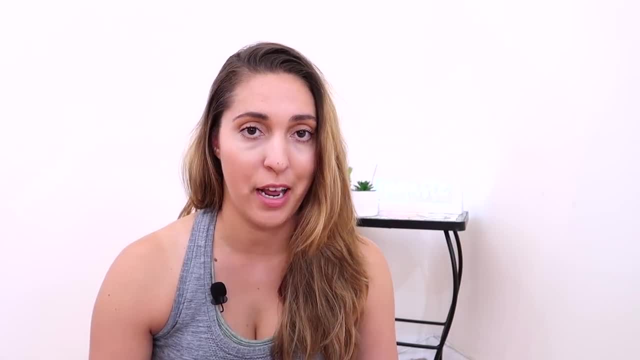 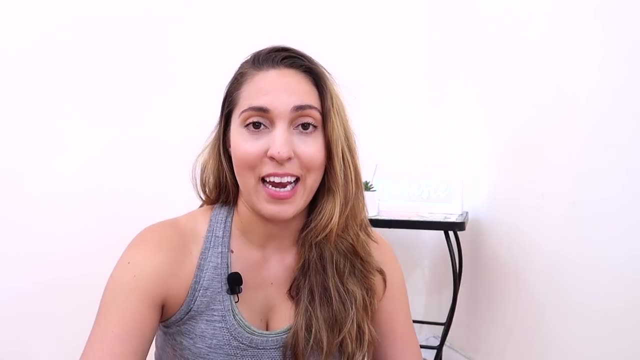 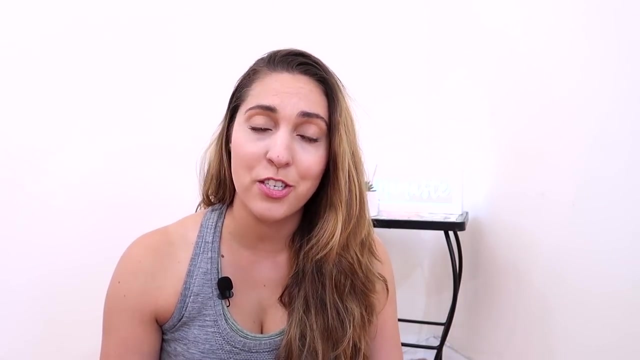 programs online are a great way to start out as well a bit more of a cost-effective option. so I hope you enjoyed those five tips and I could get into way more detail into all of the topics that I discussed, but that would be a very, very long video. so if you would like me to go into depth into any,